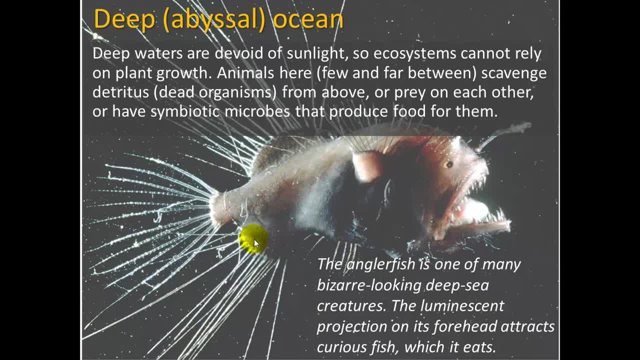 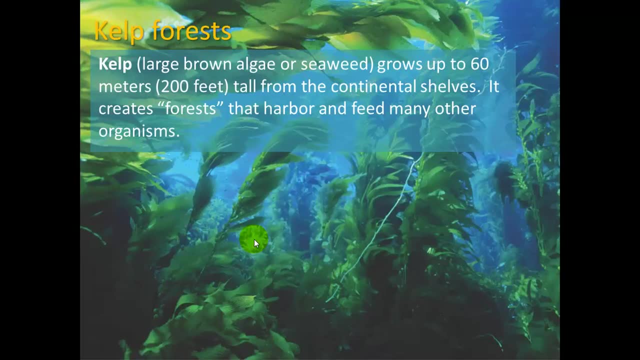 symbiotic microbes that produce food for them, And this anglerfish is one of many bizarre-looking deep-sea creatures. The luminescent projection on its forehead attracts curious fish, which it eats. Kelp is actually an algae, even though we think of it as a plant. It's a large brown algae, or often. 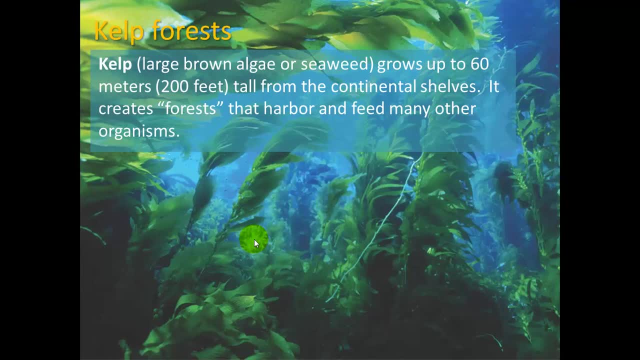 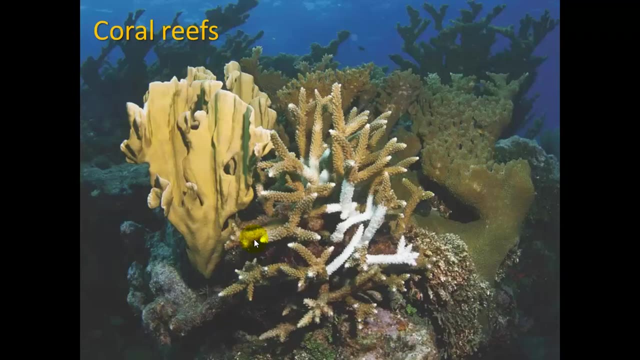 called seaweed, and it grows up to 60 meters or 200 feet tall from the continental shelves. It creates forests that harbor and feed many other organisms, And here we have coral reefs. So some significant things are that corals are. 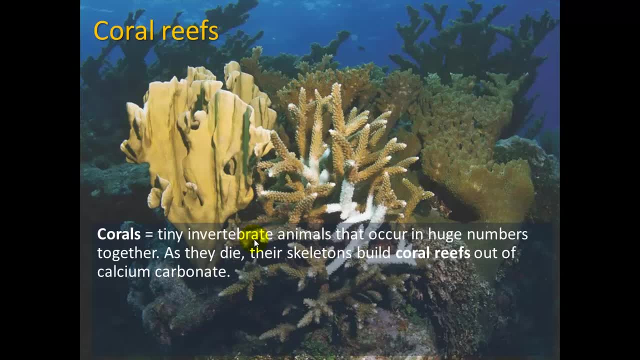 it's actually from living organisms. they are tiny invertebrate animals. Remember, invertebrate means that its structure, its vertebrate, is on the outside, whereas we, us, we are vertebrates. So they are those they are. we have our. 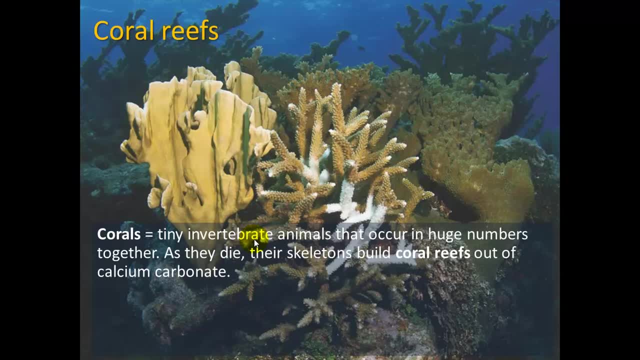 vertebrate on the inside, I mean interskeleton. invertebrate has outer skeleton. Okay, so what about them? They occur in large numbers together. As they die, their skeletons build coral reefs out of calcium carbonate, And reefs provide habitat and food for many other. 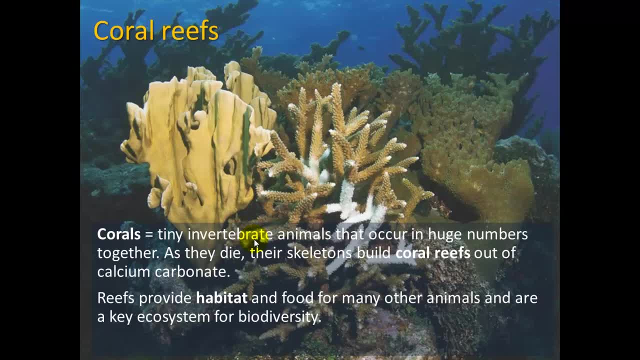 animals and are a key ecosystem for biodiversity. Okay, let's go to the next part here. They also help protect coasts by absorbing wave energy, And here we see partially bleached coral. Bleaching occurs when the algae components die And we see really colorful coral. that's from the 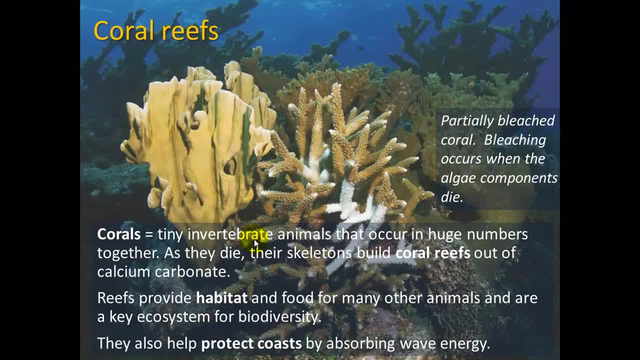 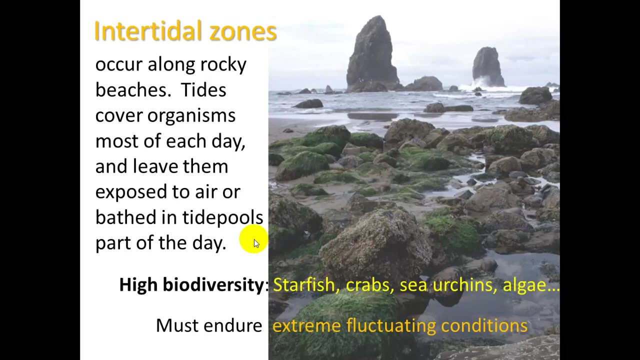 different colored algae that lives in like a symbiotic relationship with some of the other things that we're talking about. There's little things called polyps, and those are the invertebrate animals, Intertidal zones like what we see along the beaches here or at UCSB by the Marine. 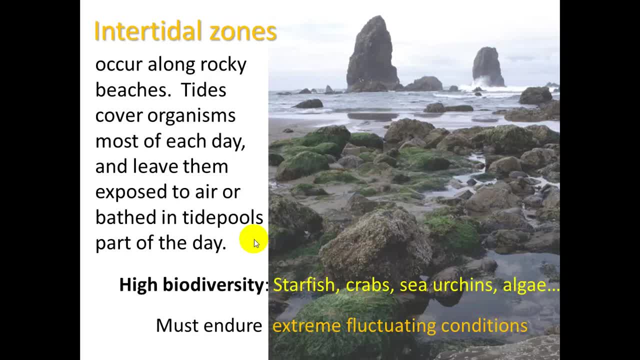 Science Institute they. they occur generally along rocky beaches where you actually have little tide pools that can form And the tides cover organisms most of the day and leave them exposed to air or bathe in tide pools part of the day. 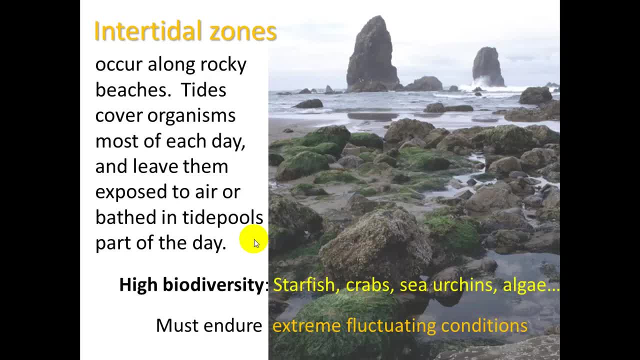 So it's really a really interesting ecosystem because you have you have creatures who need to be able to survive being submersed in water for half the day and then exposed to air for half the day or or a quarter of the day. 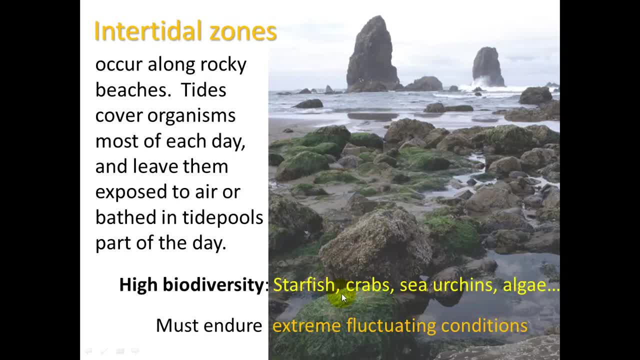 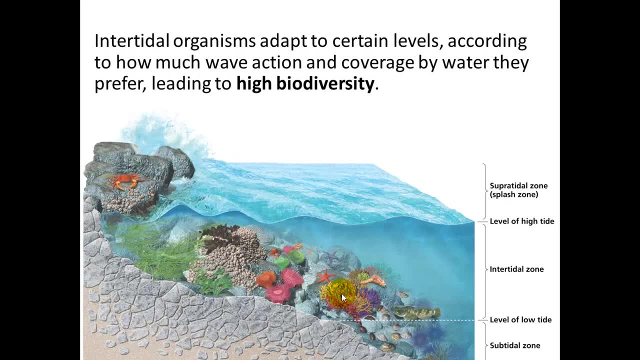 So very high biodiversity here. We get starfish, crabs, sea urchins and algae And, as we said, they must endure extreme fluctuating conditions. Intertidal organisms: they can adapt to certain levels according to how much wave action and coverage by water they prefer. 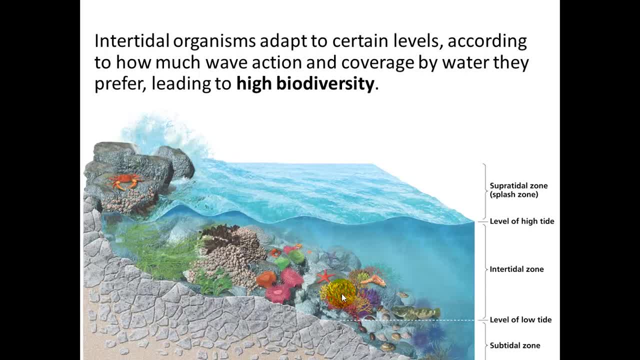 And again leading to high biodiversity. So even within these intertidal zones we have different levels. We have some zones that are generally more often um uh underwater and other areas that are more often exposed to air. 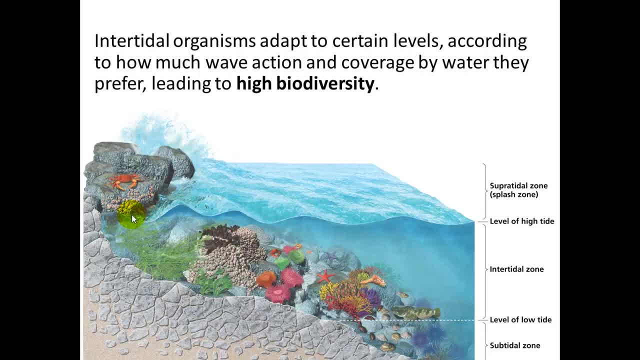 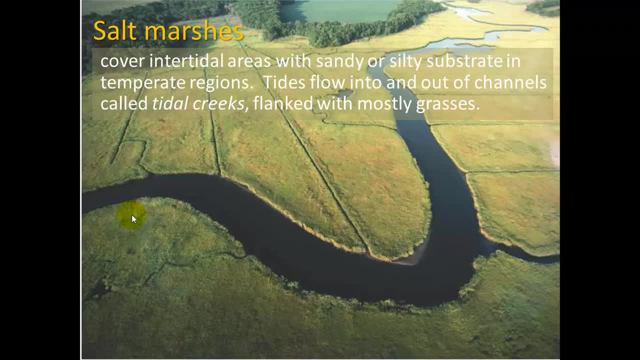 You can see these mussels along here. So even just within the span of a few meters, you actually have quite a diversity of um of conditions. Salt marshes: they cover intertidal, intertidal areas with sandy or silty substrate in temperate regions. 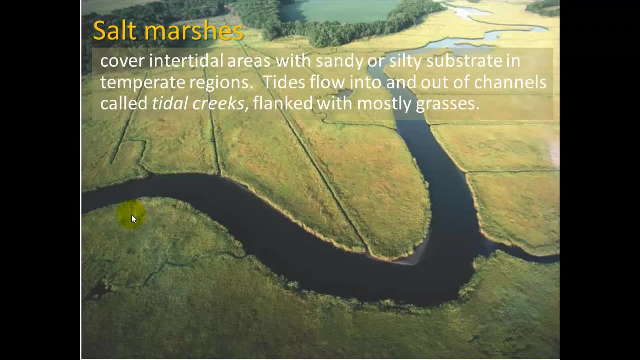 Salt marshes. they cover intertidal, intertidal areas with sandy or silty substrate. in temperate regions, Tides flow into and out of channels called tidal creeks, flanked with mostly grasses. You see this a lot in Florida. I used to live in Pensacola, Florida, or at least my parents did. I'd go visit them during college. 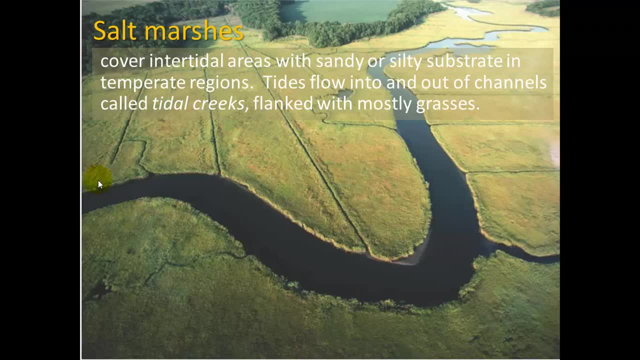 And, uh, you would drive by just miles and miles of this stuff And it would actually smell. kind of like you could smell the methane, the natural gas being given off from the anaerobic bacteria in some of the stagnant water. 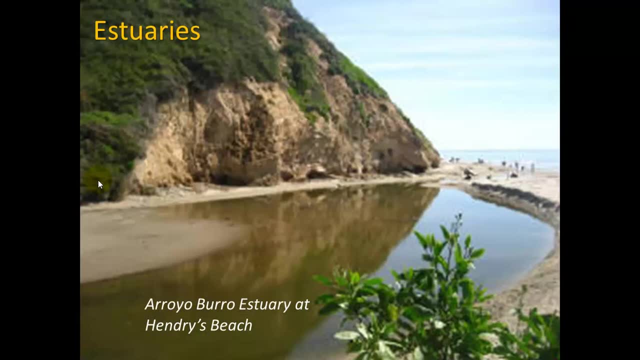 And we have estuaries. This is our local estuary at Arroyo Borough, Hendry's Beach, And these places are known for having um well, by definition, they are areas where rivers flow into the ocean and mix fresh with salt water. 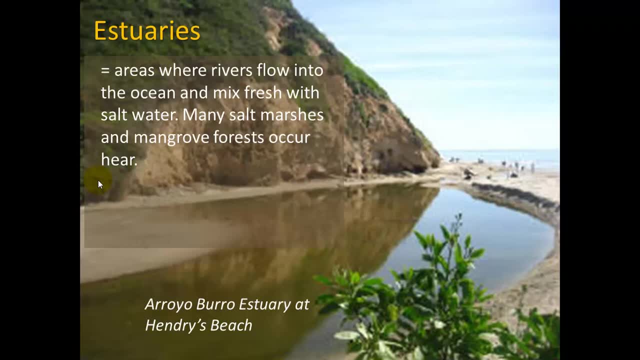 Um, mix fresh water with salt water And uh, many salt marshes and mangrove forests occur here. Biological, they are very productive. There's lots of nutrients, lots of fish, lots of birds, lots of invertebrates. 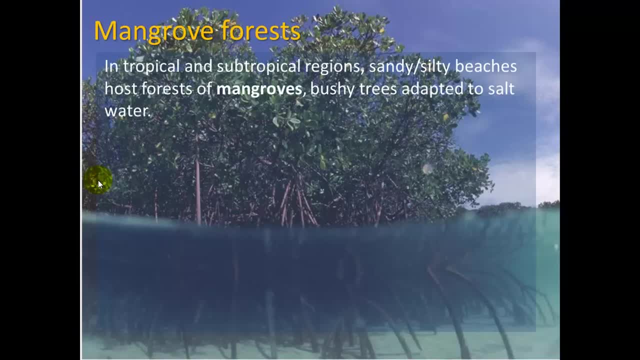 Mangrove forests. we see these often in Florida. They're in tropical and subtropical regions, sandy and silty beaches. They host forests of mangroves, which are bushy trees adapted to salt water. They're important for habitat because many animals find homes among the root networks. 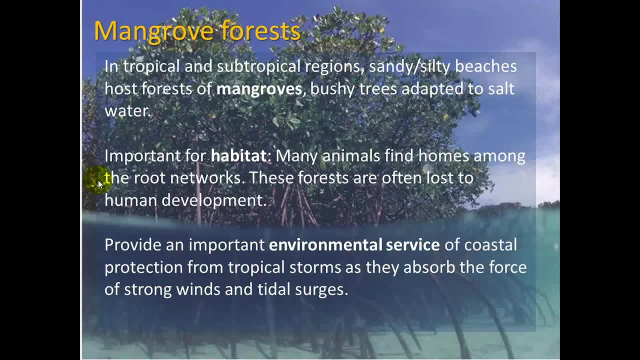 And these forests are often lost to human development. They provide an important environmental service of coastal protection from tropical storms, as they absorb the force of strong winds and tidal surges. It is said that the intensity of Hurricane Katrina, one of our worst hurricanes ever, would have been drastically improved.